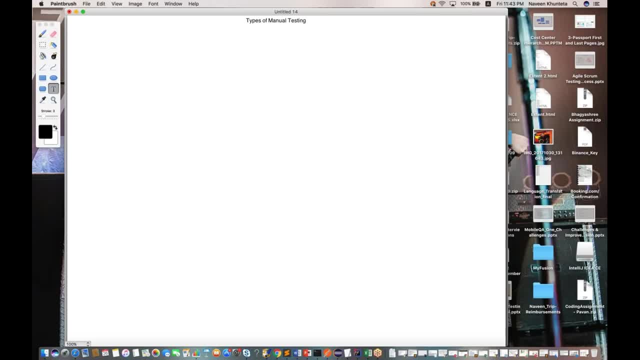 manual and automation. Very straightforward definition. is that actual versus expected? What are you expecting? And the same thing you can see on your application. It means your test case is passed. It means you okay, this is what you are testing. It means that 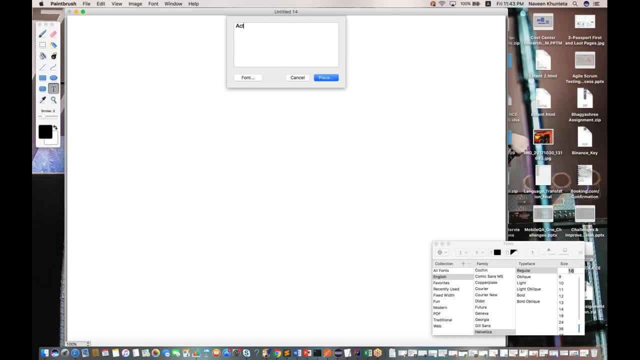 your test case feature is working fine. So testing is always. remember, guys, very short, is that actual versus expected? Okay, actual versus expected is called testing. Now, how to verify actual versus expected? there are different ways of testing. Okay, so there. 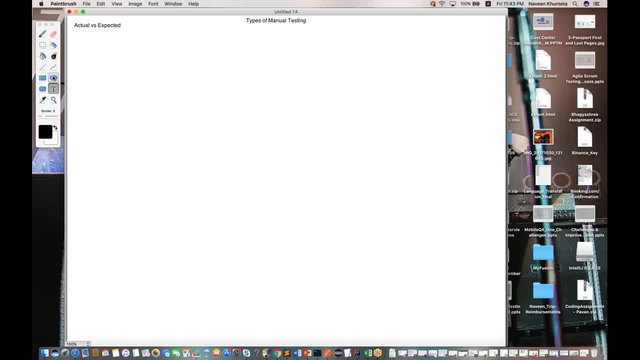 are different ways of fun. There are two types of testing. Generally, I would say, if on top of that, if we have testing, okay, so for testing, let's see it's over here. So testing is again having two parts: One is functional testing And another one is non functional testing. 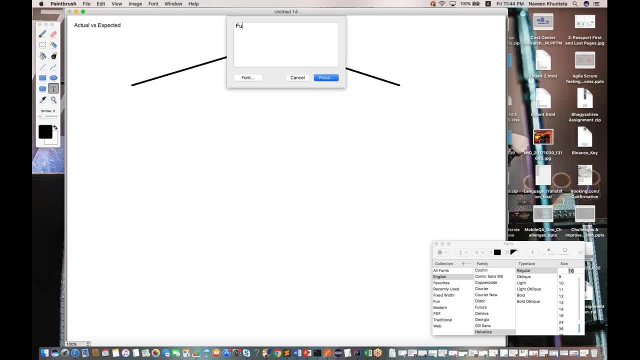 So let's talk about first functional testing. Okay, Functional testing. Now, what do you mean by functional testing? function means you are just checking the functionality of that particular application in a different way. Okay that you are checking the login scenario, we're checking the registration scenario, you are checking some the payments. 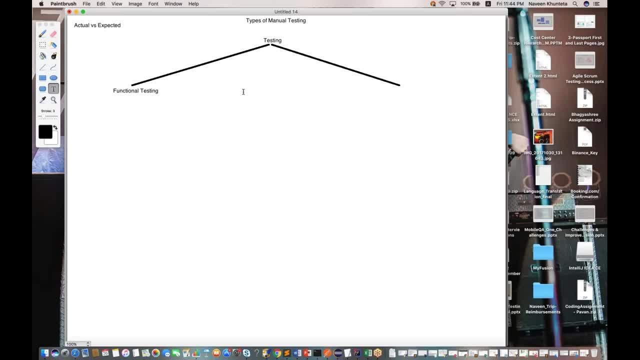 and are you? you know each and every use case and the test case: the feature wise, the functionality wise. okay, according to the requirement document, according to the acceptance criteria, if you're using sprint, okay, on the basis of that, you are writing your test cases. But those test cases, 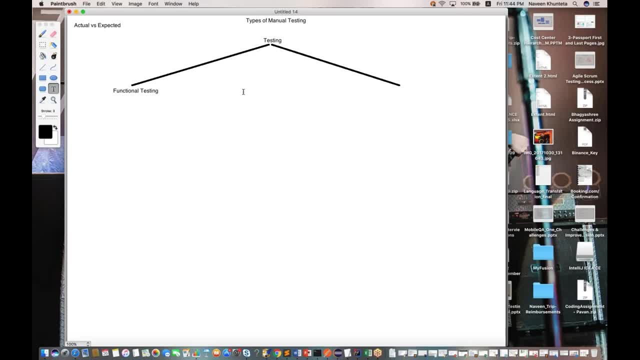 are fully functional test cases. Okay, functional testing means your feature testing. Okay, what kind of business it is. what kind of use cases are there? what are the different high level Okay, scenarios and tests. Scenarios and test cases are there. On the basis of that, you are doing testing That. 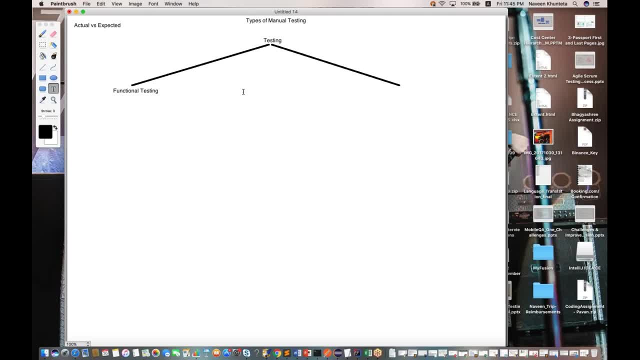 type of testing is called functional testing, where you are checking the functionality of the application. Now, functional testing is again is divided into multiple parts. Okay, So different type of testing that we have. if you write that working the, let's see first. 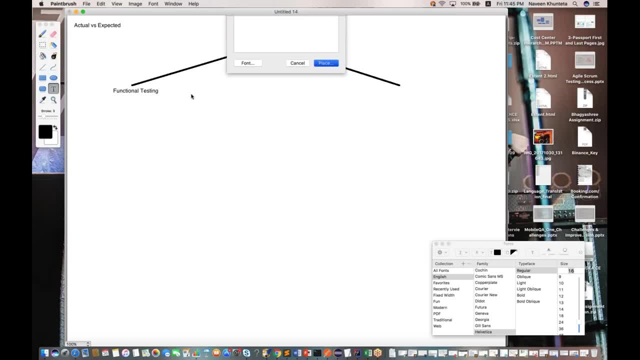 we have system testing. Okay, now what do you mean by system testing? System testing- again, it's coming under Functional testing. So system testing means the overall system. you are checking that end to end full flash system. you are checking data, number of components combining together. 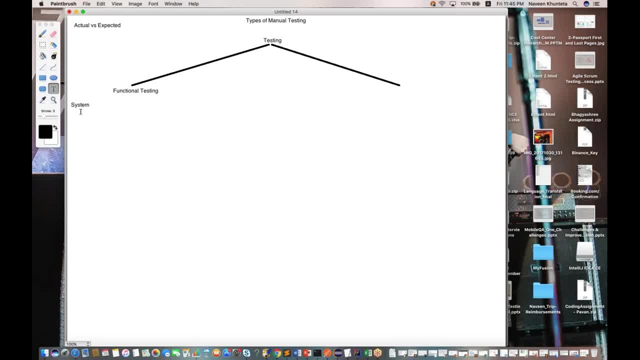 and let's see: login is a different component, Search is a different component, Home is a different component, Product is a different component. How exactly all these components are interacting and working together as a system. That type of testing is called system testing. 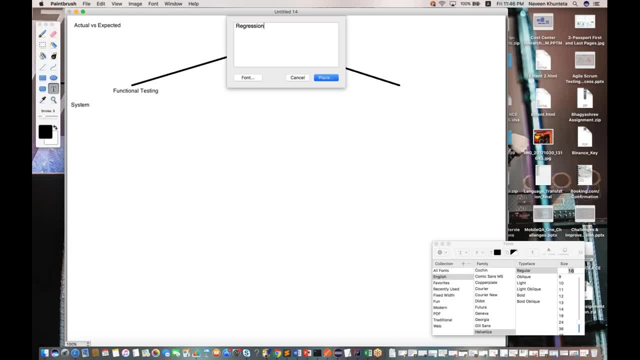 Now the most important testing is that is called the regression testing. Okay, So this is the regression test. What do you mean by regression? Regression generally, we use that. Okay, It's our daily, routine activities. that regression means whenever let's say some. 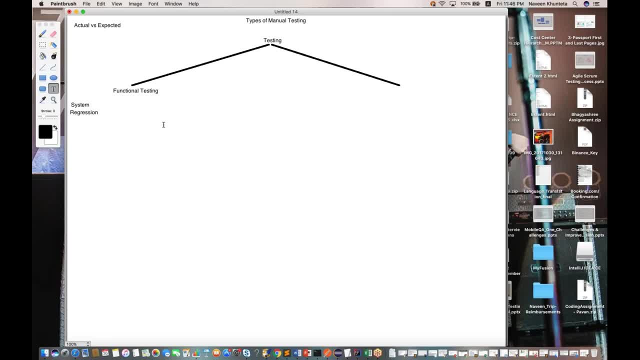 application is already already built and what exactly you are doing that? Okay, You have found 10 issues and developers they are fixing those issues, 10 issues- And now they have given to you that, okay, this is done, Although 10 issues are got fixed. And then now, please. 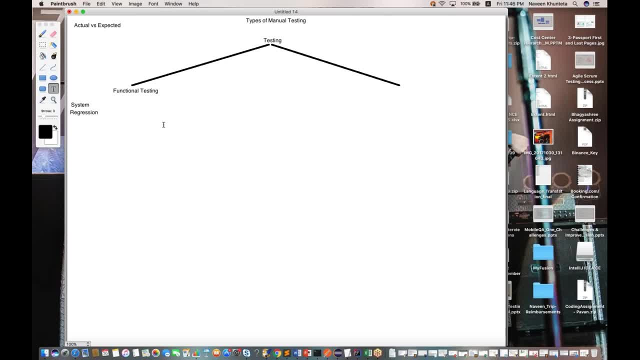 test it, verify it. So what exactly you are going to do that? Okay, You are going to test. Okay, So you are going to test the application. you are going to test the application, you to do that. okay, you are just checking those 10 issues. no, you are verifying those 10 issues along. 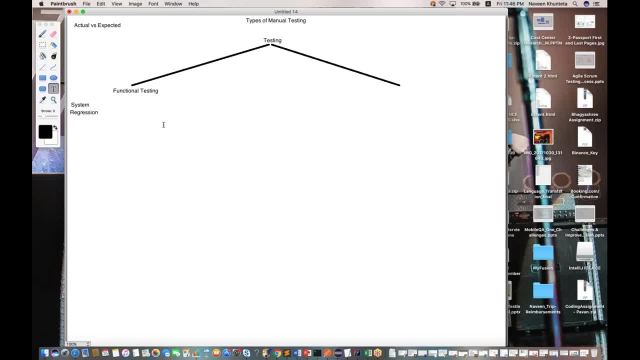 with you are checking that, okay, might be possible by after fixing of those issues. there are some issues in the application in some other areas. right, there are possibility, there are high chances. this is just like if you are doing an operation for for a brain, you are checking the complete. 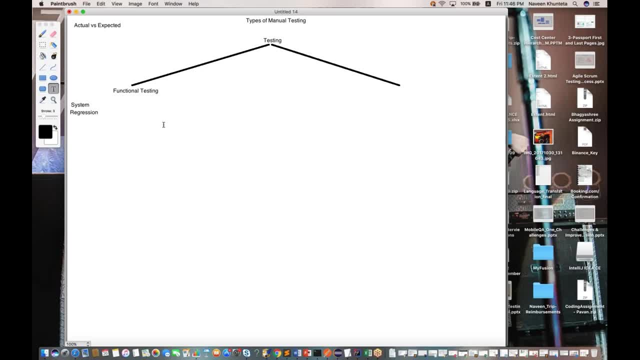 system, complete body, that okay. there should not be any leakage. there should not be any damage in some other part of the body. same thing: if any bug fixes are there in, let's see in home page or maybe some feature got fixed or maybe some new feature got added. 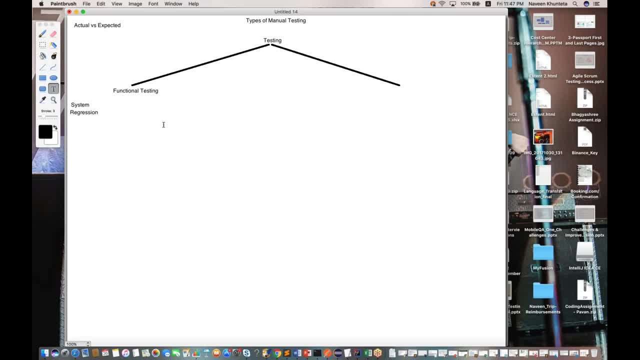 maybe because of introducing of the new feature of fixing of those bugs. okay, some other parts of the application should not be disturbed. okay, it should not hamper, it should not disturb other part of application. so that type of testing is called regression testing. apart from that, have retesting. okay, what do you mean by retesting? retesting means only bug verification is called. 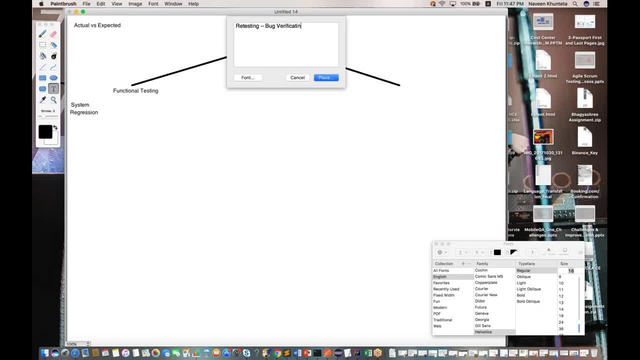 retesting. whatever the bug you are verifying, that is called bug verification. okay, that is called retesting. so retesting is just: we are just checking 10 issues. bugs got fixed. you are just verifying it that okay, these issues got fixed or not. but due to fixing of those issues, 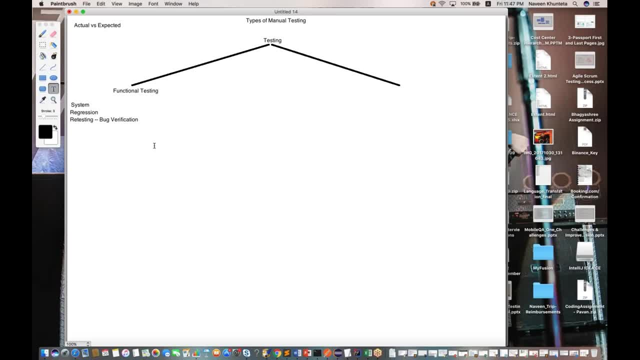 you are checking the impacted areas also. that is called regression testing. okay, then we have smoke testing. smoke testing means we are just checking, very you know, the basic feature, basic functionality, very basic feature functionality. okay, it's not a complete regression testing. let's see, the login is happening. 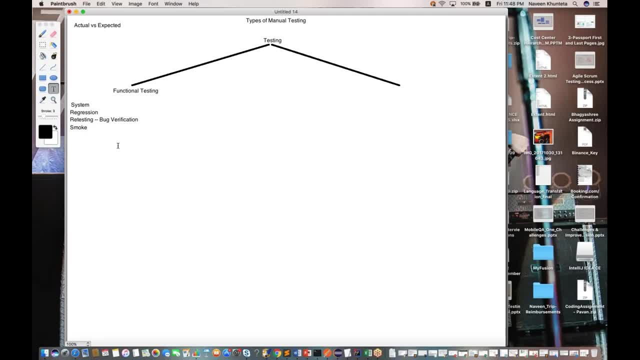 all the links are working fine, all the buttons are working fine, the look and feel is fine. okay, there are okay some basic testing. you are doing in the smoke testing. you're just checking very high level, very, very high level, that okay. yes, this particular application is looking good, the build is looking good. okay, like that. after that we 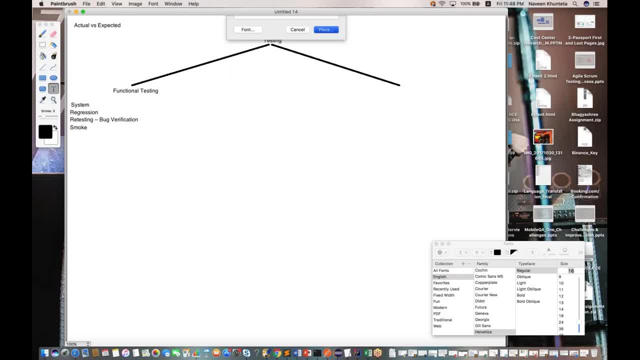 have sanity. so what do you mean by smoke and sanity? sanity means it's little advanced. okay then, smoke testing, insanity testing, that we are checking most of the high level scenarios. that login is working fine, all the buttons are clickable. okay, we are all the page navigations. 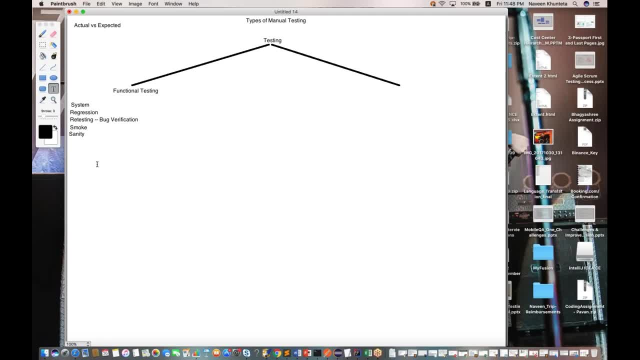 are working fine. i'm clicking on this particular button. the next page is coming properly or not? the very, very high level business scenarios are working fine. that is called sanity testing. that, okay, logout is happening properly with the different users we are able to log in- okay. that kind of testing is called basically very basic, uh, but with some high level scenarios. 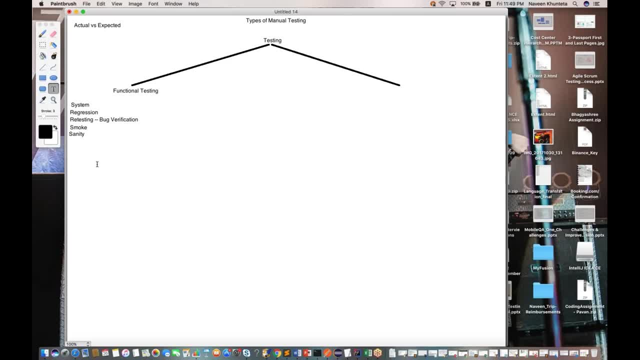 we are checking. that is called sanity testing. then we have unit testing. unit testing is always generally done by developers. okay, unit testing means on the basis of code, whatever the code they have written. okay, they are responsible to write the unit level test cases. okay, so, whatever the code they have written which is done by the developers, so whenever they are, 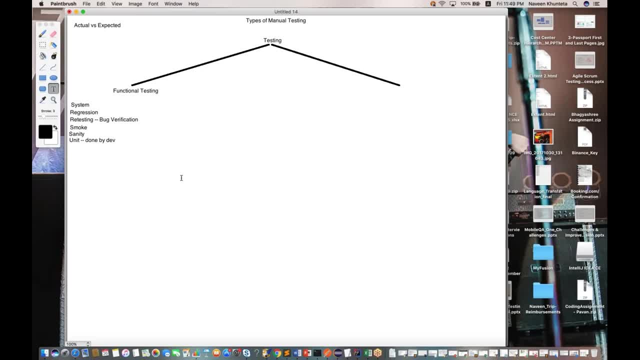 giving a build to the qa team. it's their responsibility that okay, at least first test, test the application by yourself and then, once you feel that okay, yes, it can be okay, we can give it to okay to the qa team. so that type of testing is called unit testing, that it is done by developer. 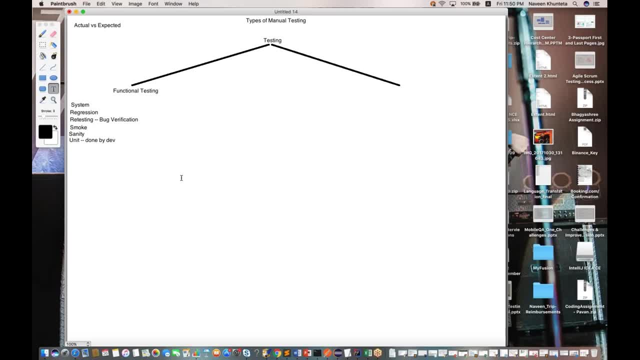 qa team, okay. apart from that, we have integration testing. integration testing means that two components, okay, are working fine. let's see, payment team is there and order management team is there. you have to, okay, interact with, okay with these two components. that type of testing is called integration testing. the two systems are integrating? okay. in that case you have to. 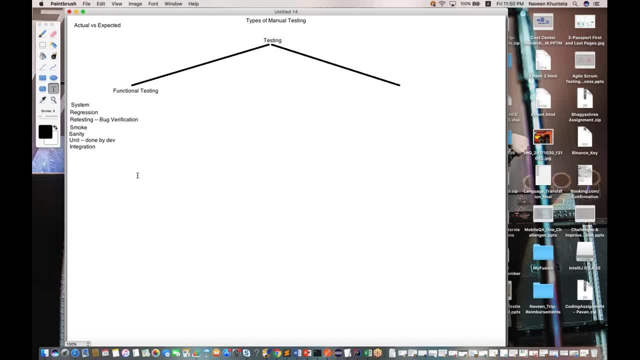 okay, check the. let's say, you're working in ola uber. so for uber we have consumer app that we are using, and then the same app, driver app, is also there. so these two systems are there, two components are there: driver app and the user app- consumer app. 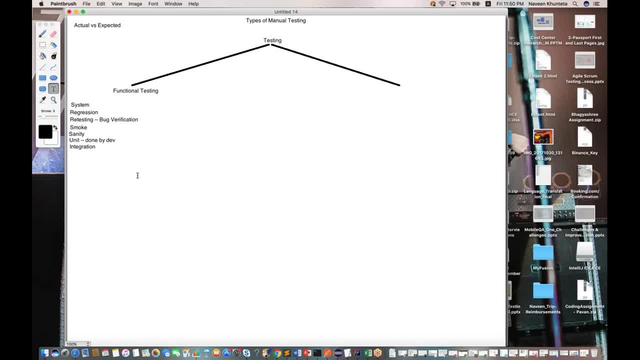 so if i'm, if i'm the qa guy in ola, i have to check that. okay, these two systems. if i'm as a consumer, if i'm booking a ride, okay, immediately the notification is sent to the uh, to the driver app, to the driver and all the driver information. the consumer can see those. 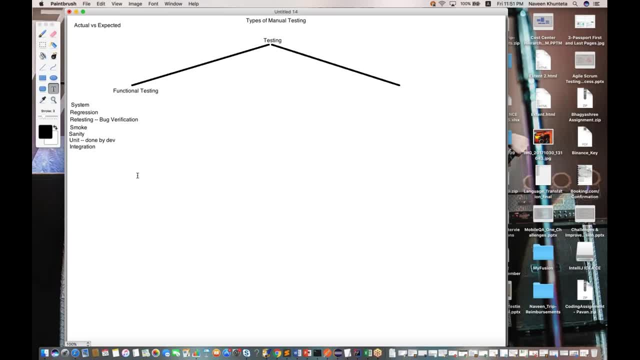 right, the information is getting transferred between these two systems, so that type of testing is called integration testing. okay, sorry, after that we have: uh, okay, integration testing is there. then we have database testing. you can say that, okay, so you are checking the complete database. that okay, uh, the database, uh, whatever data, point of view and schema. okay, all these, uh, the data is. 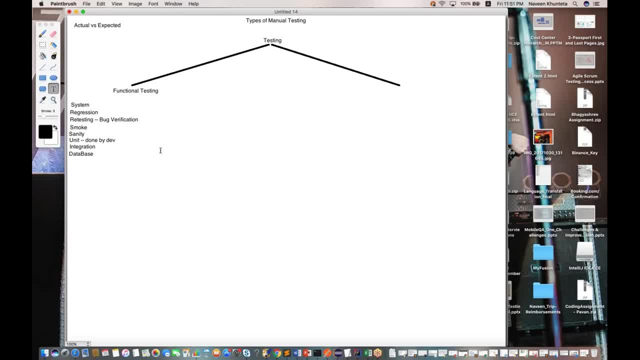 getting entered into the databases. in the proper table you can see that the database is getting. we are able to fetch the data from a database. okay, such kind of testing is called database testing. then we have white box. so white box is again very high level term. that i would say. white box means 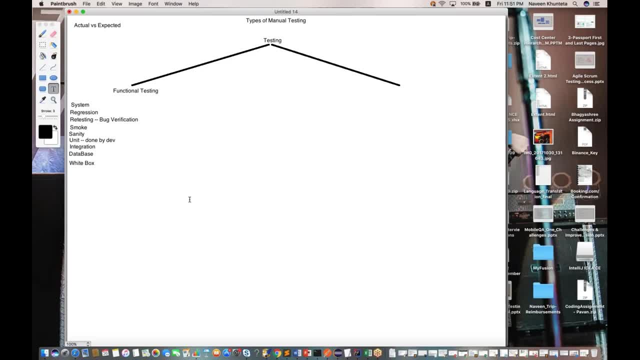 there is a, there is an application and i can check the code. i can see the code, okay, and then, on the basis of the code, i'm checking that. okay, this is what i have to test. so in white box testing, okay, in white box testing, let's see, this is, this is your box, and in this particular box, your code is. 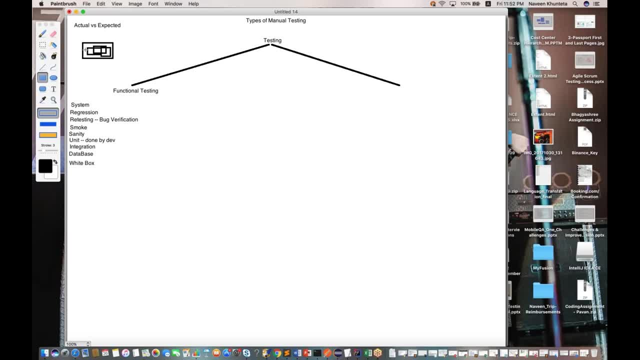 available over here. this is your code, right, so i can see this particular code. so, on the basis of code i have to write my test cases. okay, some automation i have to write, or some script or java code i have to write to test that particular code that is called white box. white box means i. 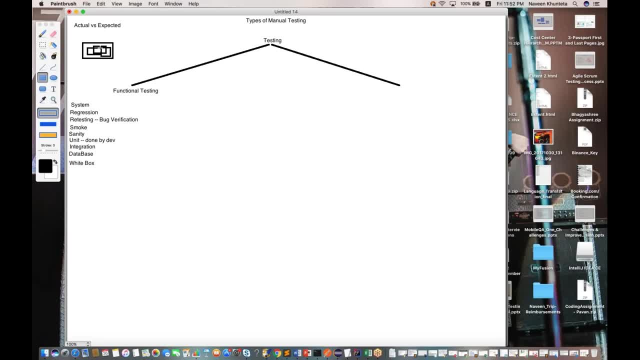 can see this particular box. what exactly inside the application? like back-end testing, apa testing. okay, the complete the code. i can check the controller, the. what kind of code? okay, the methods they have written so that i can check those methods by writing my script. okay, then we have black box testing. black box means there is simple black box. i cannot see what. 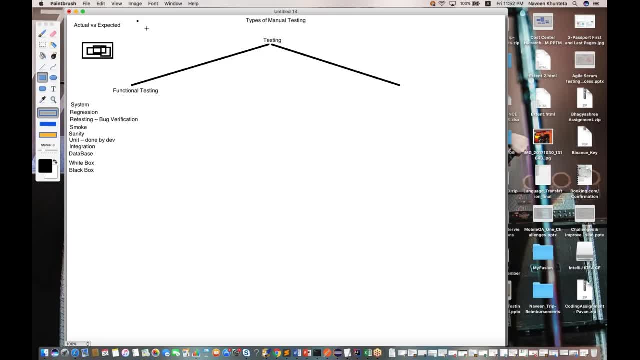 exactly it's written. okay, so there is a black box. this is a black box. i'll just pass for input and i'll get the output over here and pass the input. this is input and this is output. i'm just getting okay, passing the input on the basis of that input. 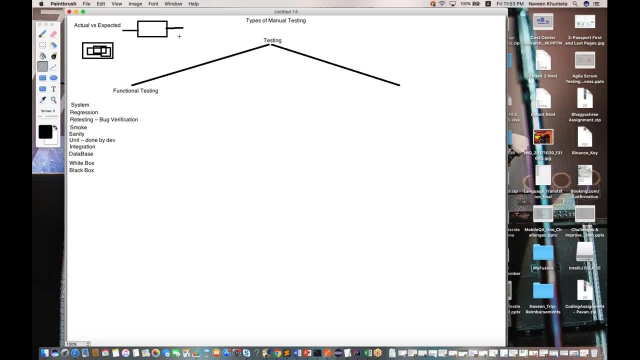 your application will perform something and it will give you the output, but i don't know how exactly it is doing, what exactly it's written inside the box, inside the application, because this is a black box. i cannot see that. i don't have any knowledge about that because i'm the black box. 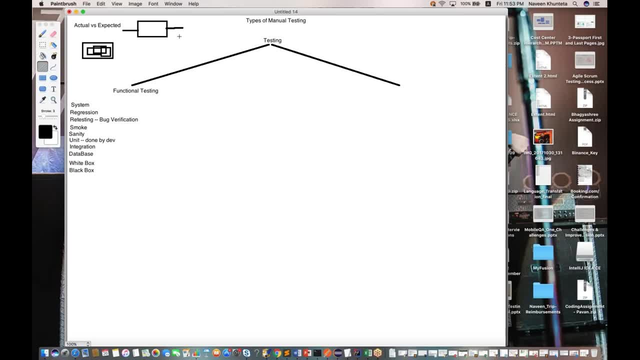 tester right, so i cannot see that i'm just passing the input and getting the expected output. if i'm the correct output, it means my test case is fast, means the feature is working fine. that type of testing is called black box testing. another one we have gray box. gray box means the black. okay. 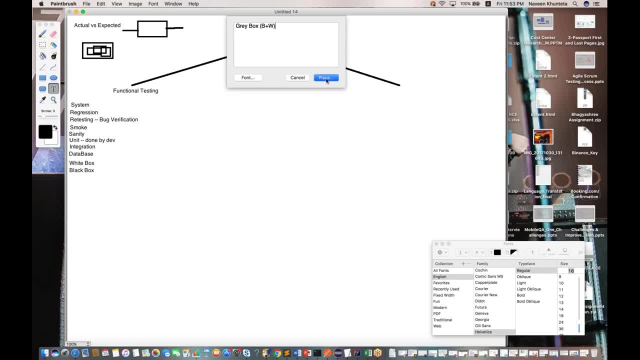 black and white box testing, both. it means i'm doing black box also and white box also. some of the component i can see, some of the component i cannot see. that type of testing is called gray box testing. okay, then we have some. you know, monkey testing. monkey testing means just like. 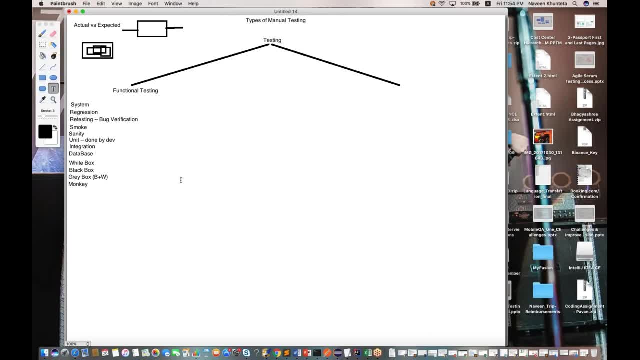 a monkey. that monkey jumps here and there, okay, randomly. so we are doing some monkey testing. that, okay, i don't have any okay time for that, for execution of the full test cases. i just play with the application, okay, and i'll check the system. that, okay, it's working fine or not, i don't. 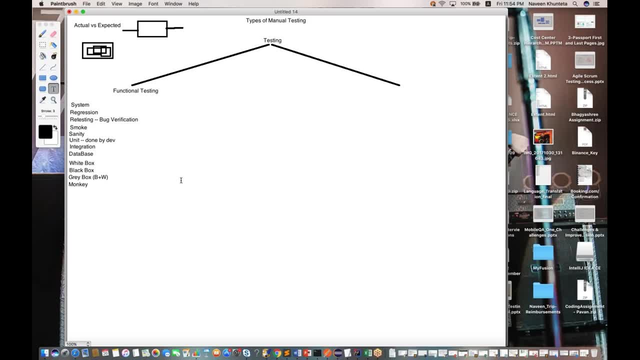 have any idea about what kind of- uh okay, things are there inside the application. what are the different features are there? let's see some. if i give you facebookcom, so i just say that, okay, you don't know what is facebook, just test it. so, according to your gut feeling, according to your knowledge and 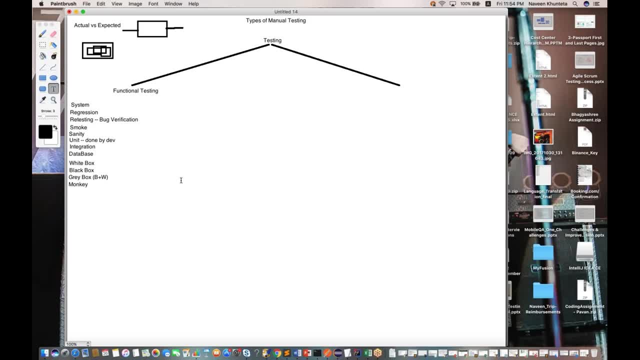 understanding point of view, you are just doing the monkey testing randomly. okay, another, very similar, is called ad hoc, ad hoc testing, ad hoc testing or maybe random testing, similar kind of monkey testing. that, okay, you are checking without knowing the application, the feature of the application, that you don't have any idea about it. okay, monkey testing somewhere you are aware about, okay, what? 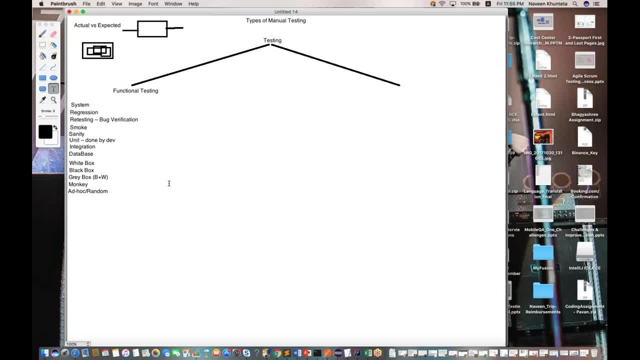 kind of application? what are the different use cases are there, okay, and what are different components out there? but you are not doing in in a proper way. you are just just like a monkey. here and there you are checking, clicking on the button, submitting the form- okay, entering the form, and. 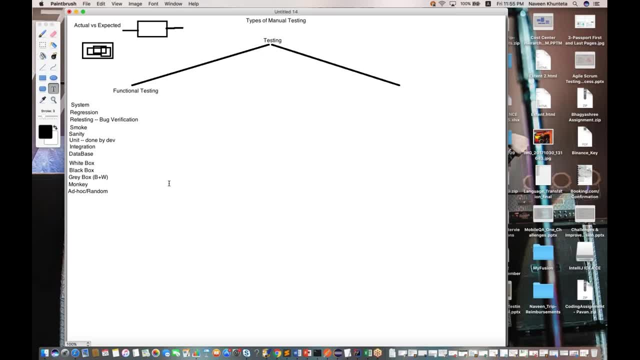 clicking on submit button and page navigation, everything randomly you are doing, but in ad hoc testing and random testing again that you don't know anything about it. so it means it's a monkey test. okay. and so when you put together your traits, that if it's your user and your particular 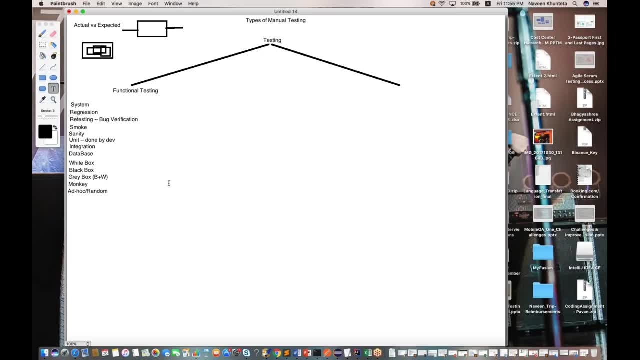 again that you don't have any idea about it and you are just checking all the features very randomly and very ad hoc, in a very ad hoc manner. that type of testing is called ad hoc testing or random testing. okay, another thing is that that is called component. okay, component testing. so what? 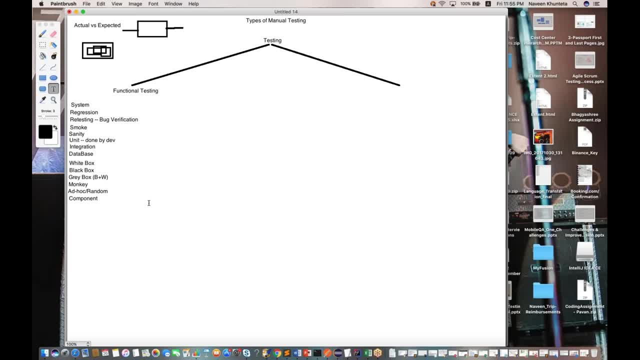 do you mean by component testing? means that the specific component, the specific module only you are checking. okay, if you integrate multiple components, that is called system testing. if you are checking only two components are working together, that is called integration testing. so component testing means: let's see, only login component is ready or let's see only payment. 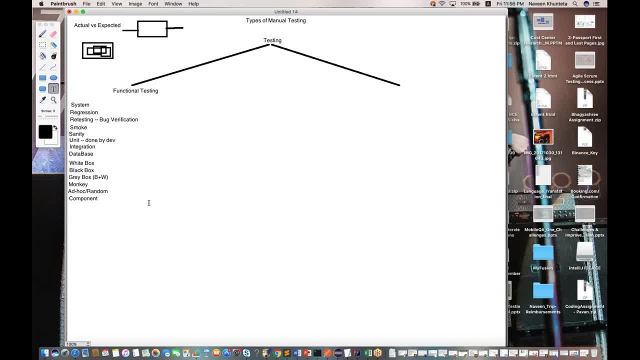 search component is ready, so you are just checking the search component. that's it, that you are able to search the product on amazoncom or flipkartcom, like that. okay, after that we have gui testing. we means graphical user interface, whatever you can see the look and feel, the alignment. okay, that images are properly. 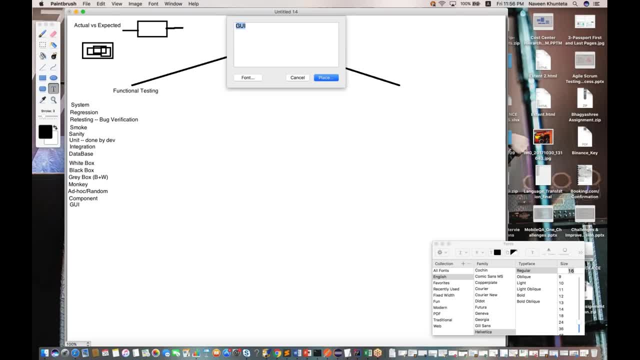 the color: okay, the design, everything is fine. there are no mismatch in the alignment. the colors: okay, button colors and all the buttons are properly aligned. the tables are properly aligned. okay, text are not overlapping. okay, the proper headers are available. proper headings are available. okay, the column names are not. um, you know, mismatching. sorting is happening. 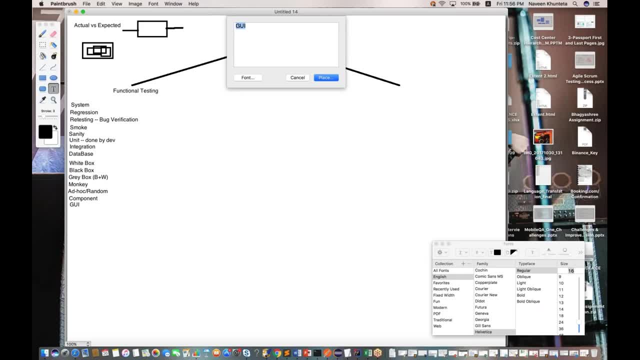 okay, the column. wise, such kind of testing is called gui testing. okay, graphical user interface testing. then we have end-to-end testing. end-to-end means a full, from launching the browser to end-to-end scenarios. you are checking the complete integration, everything. you are checking full end-to-end test cases. okay, the complete business. 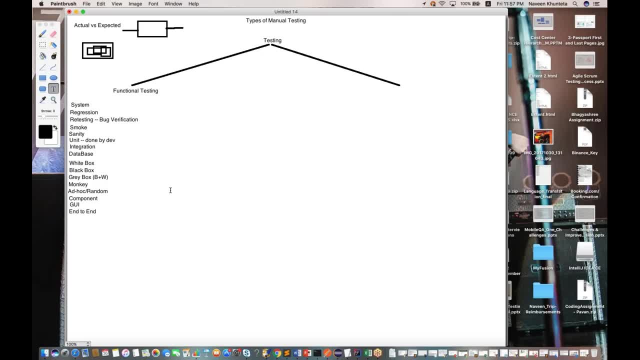 flow. you are checking, okay, from the beginning to end. that is called end-to-end testing. okay, after that, then we have uat, user acceptance testing. so in uat again, guys, there are two type of testing. that is called alpha testing and that is another is called beta testing. so in uat we have two types of testing. that. 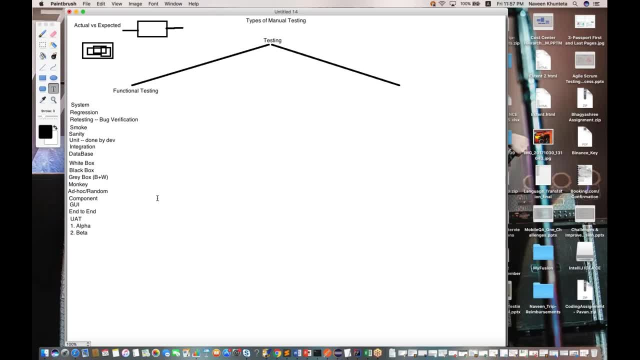 is user acceptance testing, that alpha testing. let's see we say that, okay, this particular product in beta stage or alpha stage. so in uat, user acceptance testing, let's see i'm creating a product. let's see i work for amazon or maybe some. let's see all our uber. so in uber, that. 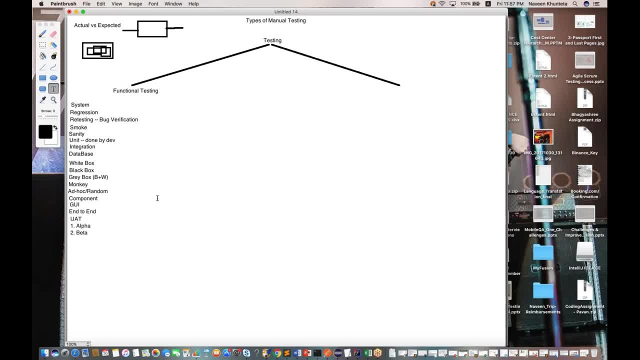 they have introduced a particular feature. so first the tester or some development team or the business people: okay, in uber they will check. okay, that whatever the feature we have given to the development team, they have developed properly or not. so let's see one guy from qa team, one guy from 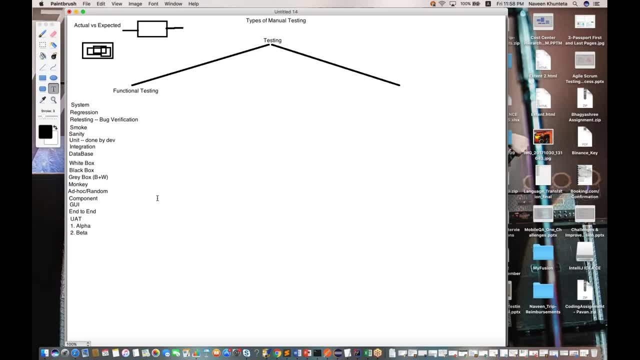 dev team or maybe business analyst or product manager. they will sit with the business, okay, with the management, management and the business holders, stakeholders. they will see the application, that okay, it's working. fine, it's ready for the production or not. that is called uat alpha testing. once this particular product will 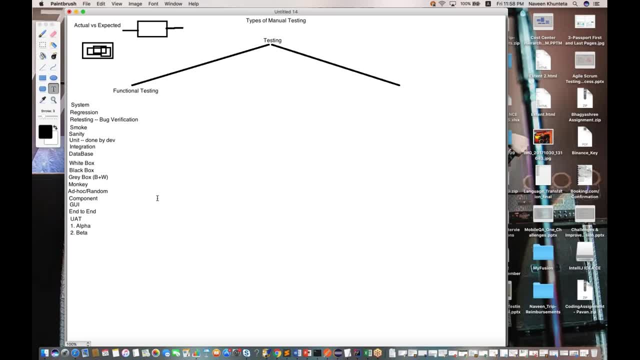 be launched in the market which can be okay, accessible by us, by the consumer, by the user. okay, and the user? let's see, i'm facing some issue with respect to uber, so i'll raise a bug in uber customer care, or maybe user uber support team or ola support team. okay, this is what we have found. 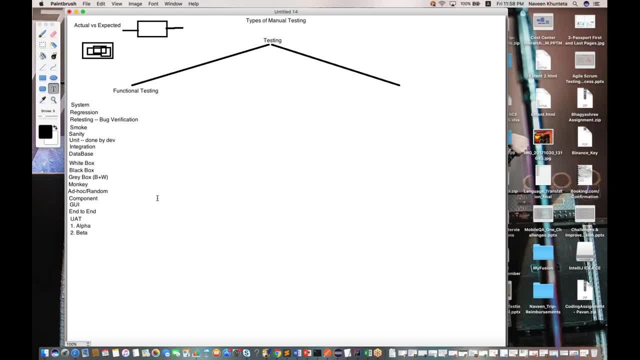 so on the basis of the customer feedback, customer is giving some feedback. on the basis of that, that type of testing is called beta testing. then the qa will be asked: okay, why did you miss this particular issue or something like that, why this particular issue is coming in the production? because that type of testing is. 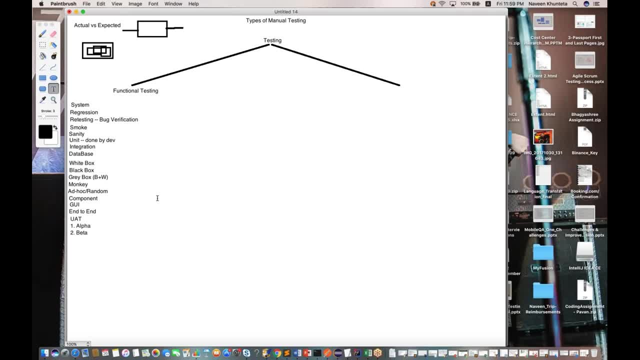 done by us, by the consumer, by the user, although we are not testing it, but with our experience, with our users, we are sharing our feedback with the customer care, with the application. okay, according to the data. also, they are checking. okay, what are different? uh, let's see some payment. 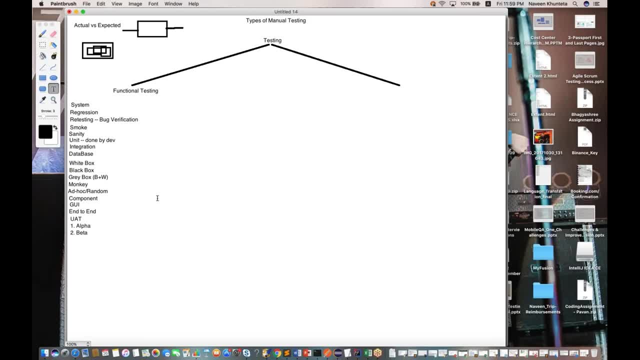 issues are there. we are not able to make the payment through wallet or paytm or something like that. maybe some integration problem is there. integration testing is not done in that area. maybe some use case is after five kilometers there are number of surcharges. are there peak time surcharges are not applicable, so it's a revenue loss for google. so on the basis of that, 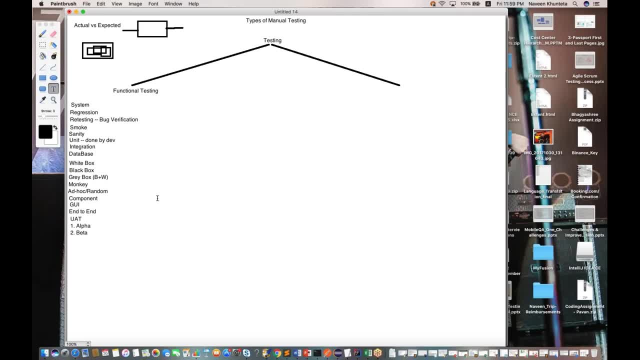 they are checking the beta testing. okay by the customer. okay, after that we have sometimes acceptance acceptance testing. acceptance testing is again very similar to that: okay, this particular uh or what are the features that you have developed. okay by the business. it is accepted in the form of alpha testing. so that is called acceptance testing. okay. 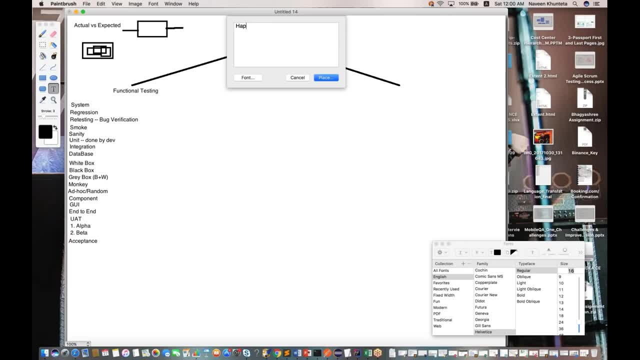 then we have sometimes only happy path scenarios, happy path testing. okay, so happy path testing means very similar, only very, very high level, very high level functionality. you are checking- okay, no, you are not checking- only negative flow. nothing that's is called happy path testing, only very, very basic flow. you are checking that is again similar to 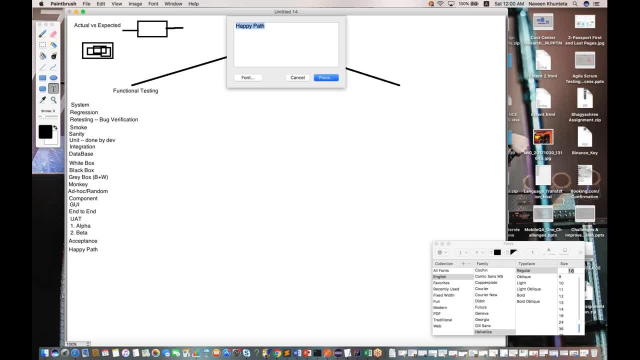 smoke and sanity testing. that is called happy path scenario. just generally we do it on production, once the production release is done. we are just checking happy path scenarios only and only positive flows. okay, that you are checking. then we have negative testing. okay, so negative testing means with the, with the at a time of system testing or maybe regression testing. you are checking all. 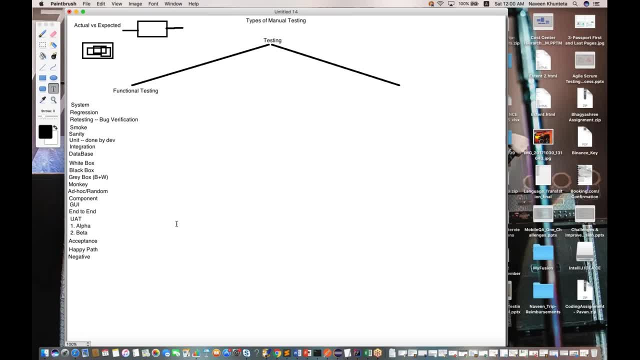 the different types of test cases like wrong value, wrong password, wrong username- okay, wrong password. you are entering blank username. blank password. you are entering null values- okay. different type of negative data. you are passing different type of different uh use cases. you are negative use cases. you are performing. that type of testing is called negative test cases- negative testing. 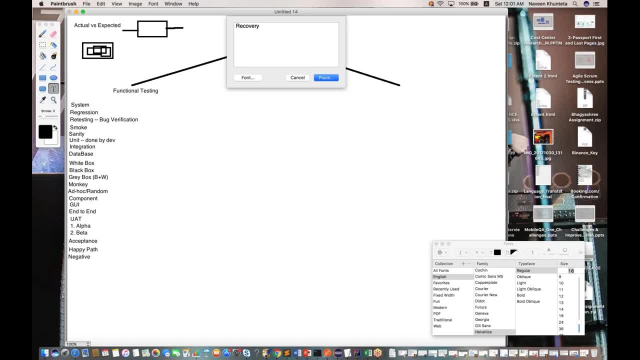 okay. then we have recovery testing. okay means that okay with the number of users or maybe some, uh, you know, application got crashed, maybe some xyz reason, so how exactly and how quickly? okay, the application is stable. the stability testing you are doing, or recovery testing you are doing that okay, uh, application is smart enough to recover by itself. so that type of testing is. 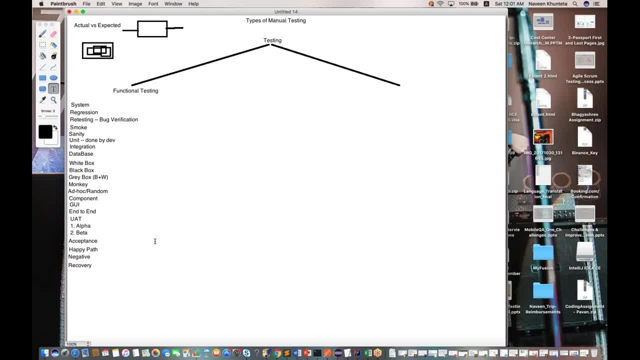 called recovery testing. after any crashes, let's see, your database got crashed, or maybe server got down suddenly or maybe it can be any xyz reason, okay, so that is, that type of testing is called recovery testing. then we have a- okay, very important- that is called static testing. so in a static testing, 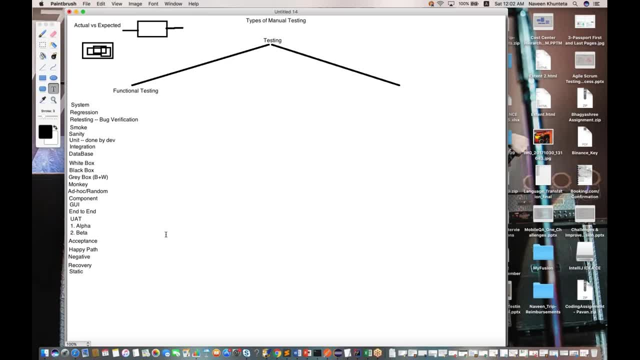 what exactly we do that? okay, without any application, on the basis of the requirement, we do static testing. that application is not at all built, very beginning, when the requirement is there, or maybe acceptance criteria is there, we are here to make the best use. if- and you have aalez горling, we are here for the scrambled. 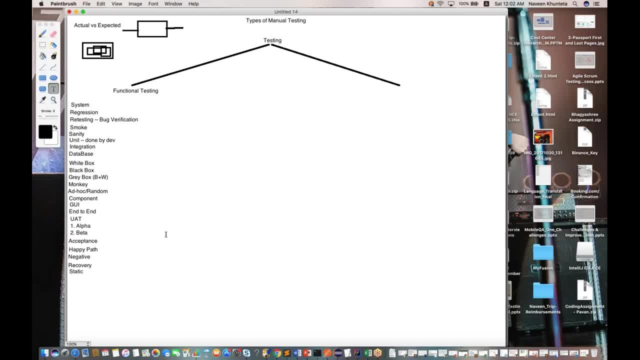 testing but we need to umm, check code. okay, we are. uh, by seeing the code, okay, we have to check the code. i mean there and there is no code. sorry, why not? by seeing the code, i mean there is code is still development, under development and not full. uh, code is not fully. 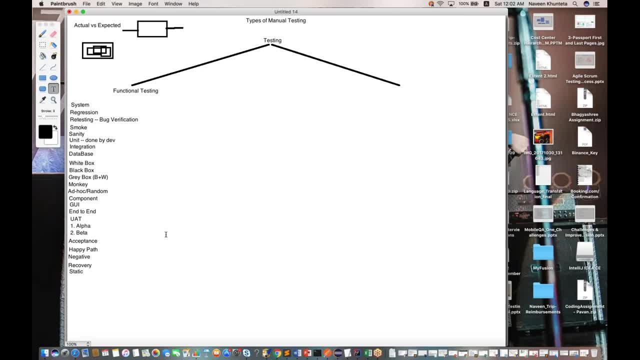 ready. in fact, it's not at all started. only requirement document is there, or maybe acceptance criteria is there. so, on the basis of that, ask you at a time of interview: reviews, walkthrough and inspection. okay, reviews, walkthrough and inspection, that is part of your static testing, so you do it. 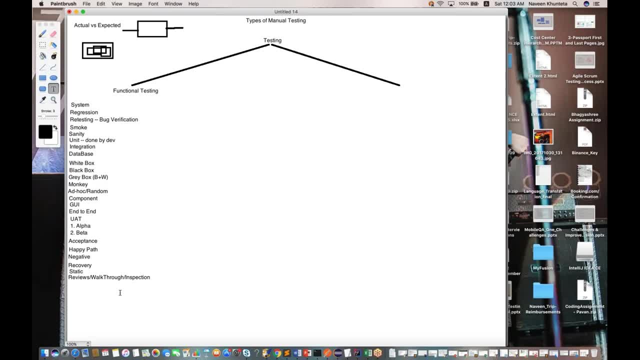 review. then it will be walkthrough, will be done by business analyst and they will do some inspection. okay, for all the requirements. that is called static testing. okay, apart from that, we have compatibility testing. okay, compatibility means the browser specific, the cross browser, that, okay, this is compatible with this particular system. okay, or this particular operating system. 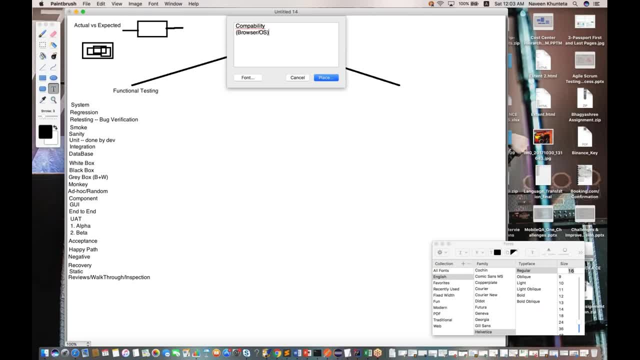 that Mac, Windows, Linux, Unix, Firefox, Google Chrome, Safari, okay, Internet Explorer, all such kind of thing that you are doing compatibility testing, okay. so such kind of thing you are doing through compatibility testing- browser specific, okay, system specific, operating system specific- such kind of testing is called compatibility testing, okay, so 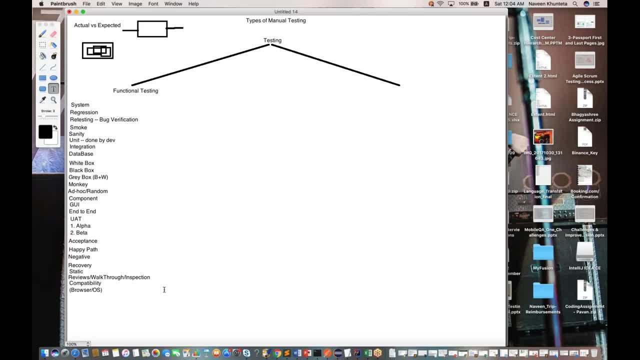 yeah, so these are different types of functional testing things. okay, now let's talk about: okay, so now let's talk about non-functional. non-functional means that you know we are not checking the functionality, so non-functional is always done. once the feature is a stable, the functionality is. 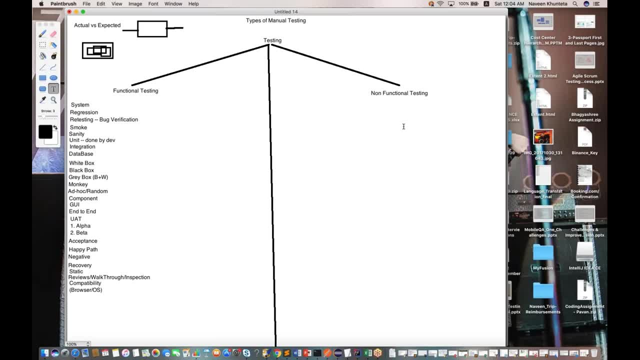 working fine, that all the functionalities are work perfectly working fine, that you have done all these such type of different types of testing and there are no bugs in the application. everything is fine. application is very, very stable. then we have to do some non-functional testing. that non. 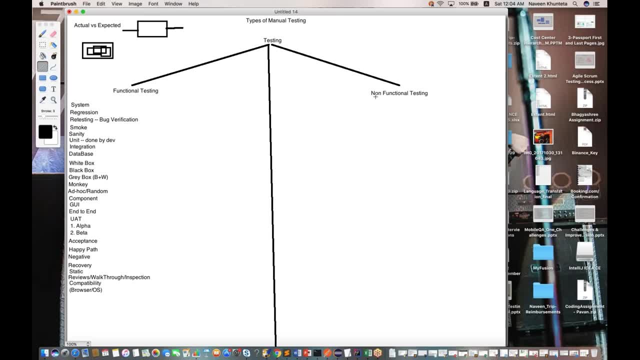 functional testing. again the major role is that is called a non-functional testing. that is, again we have performance testing, we do performance performance. okay, in performance testing we do. we are checking the performance of the application with a different load. let's see thousand or ten thousand or 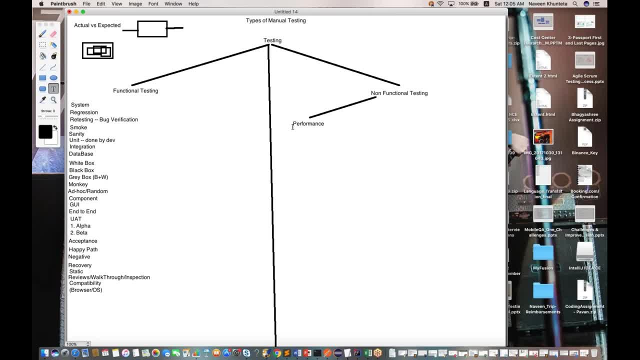 millions of users are using uber app amazoncom during holiday season, during Thanksgiving Day, during Christmas season, during Diwali season. we are hitting that particular Amazon application. so you are checking the performance of the application. that, okay, the Amazon server is able to handle the data, handle the. 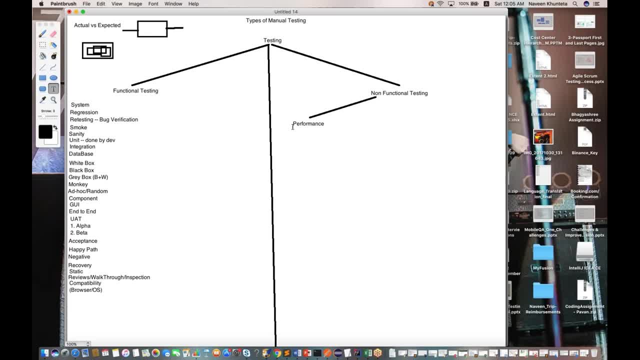 such kind of huge amount of request or not. that type of testing is called perform and testing and performance. also it's divided into multiple partnership load testing load means we are checking with a different load, with single user, with 500 users, with 5,000 users. what is the response time? how much? 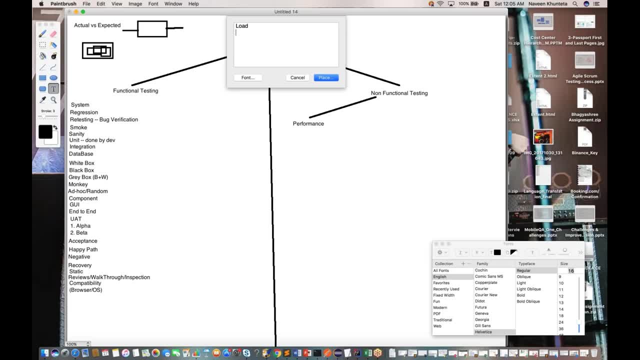 time it is taking to okay get the response. what are different? ok, memory leakages, CPU utilizations: are there? such kind of testing is for load testing. then we have stress testing. we are checking the threshold value. ok, let's see one ok bulb is there, or maybe a tube like. 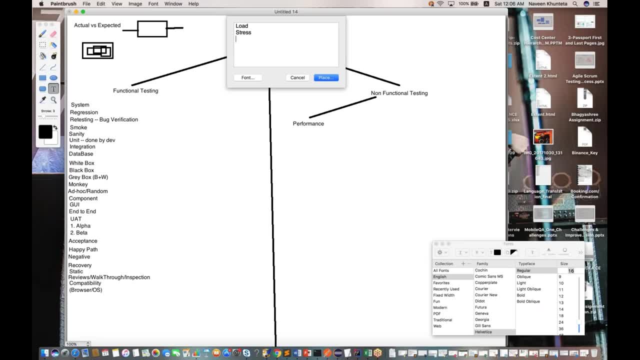 this and we have stress testing. ok, then we are checking the threshold value. ok, let's see one ok bulb is there, or maybe a tube like this: is there the maximum? let's say it's a 60 watt bulb, but you are increasing the watt. let's see: 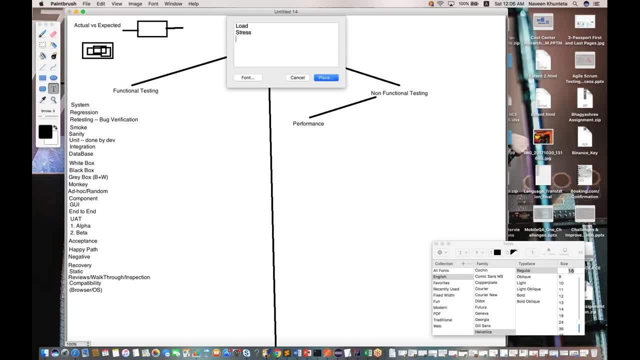 a 40, then 50, then 60, then you have reached to 70, and then 80, and after 80, suddenly you see that okay, bulb got crashed. okay, the same thing you are doing with the stress testing. that okay, maximum at a time. you have to benchmark. you have to do some benchmarking, that okay. 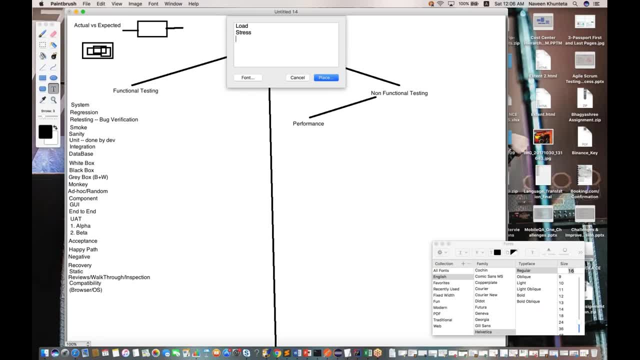 after 10 000 users. my server will be down at a time. so you will do some stress testing. you will give so much amount of load at the same time, you know, to the, to the server, to the, to that particular site, and then you will check the performance of the application, how exactly it. 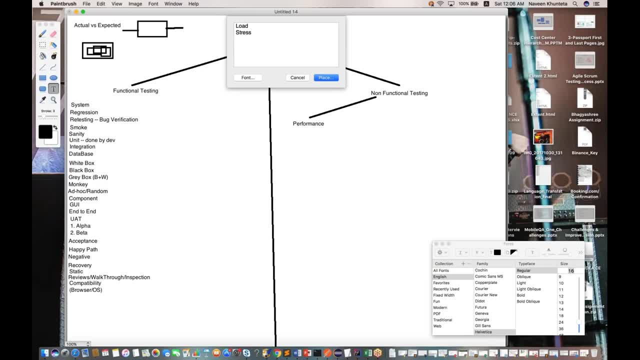 is doing. okay, so you will check the threshold value, what exactly the maximum limit of load, maximum amount of load this particular server can handle. that kind of testing is called stress testing. then we have volume testing. okay, volume testing is again similar to load testing. you are checking the different volume. okay, that how many resources are getting utilized with this particular. 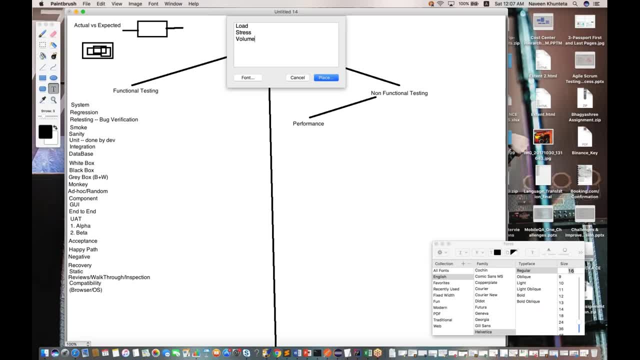 500 users or 5000 users, okay, like that. so you are checking that with a different volume, with the different threads you are passing and checking what exactly, how exactly application is responding. so that is called volume testing. base on all these part of performance testing, now we have 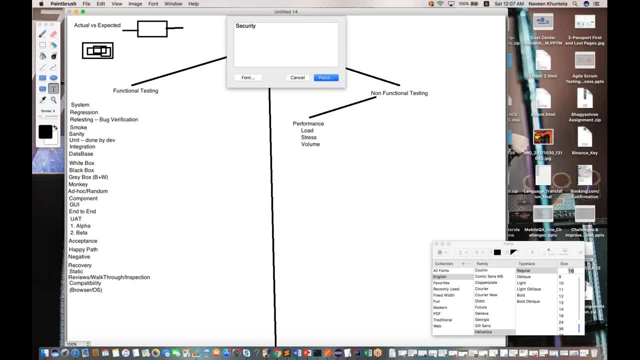 a security testing in, uh, okay, in functional testing we have another thing is called security testing. so security testing is again. obviously, once the application is stable, everything is fine okay. so you are checking all the options. that okay, uh, uh, you know, penetration testing. you are checking, okay, penetration testing. is there sql injection? 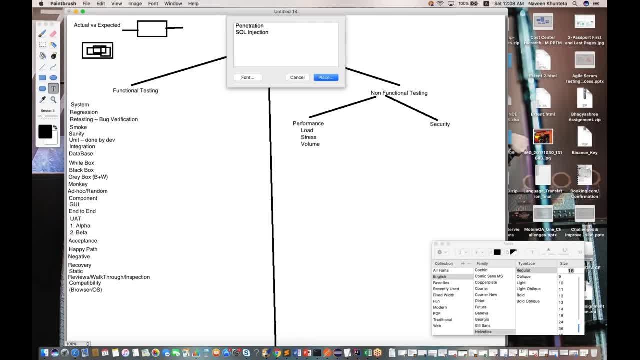 or you are passing some sql injection in the username password field on the ui. let's say i'm passing select a star. okay, select a star from user table where username is equal to navin and select password. let's see i'm passing select password from employee table where employee 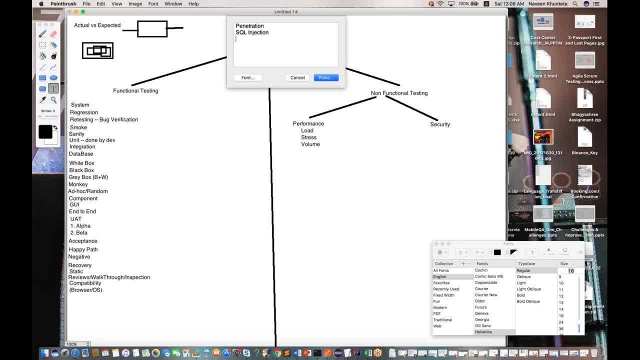 name is equal to navin. if i'm getting the password, it means i'm through sql injection on the ui, i'm getting the password, i'm able to hack your application. okay. so such kind of sql gallons in that way is all enabled by sql injection. run write connection is equal to navin. we fix now so we take those languages. 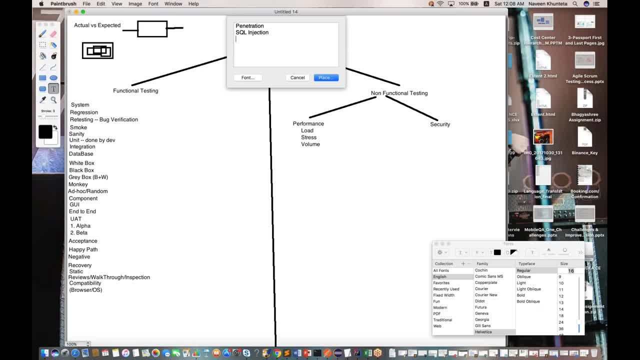 sql injection on the ui. we are neglect of mist configuration. sweet ***. use sql injection of infrared vaya так as, when done, able to hack your application. okay, so such kind of sql injection we will pass. so all the sql injection should be avoided. it should not accept. so it's developer's responsibility to. 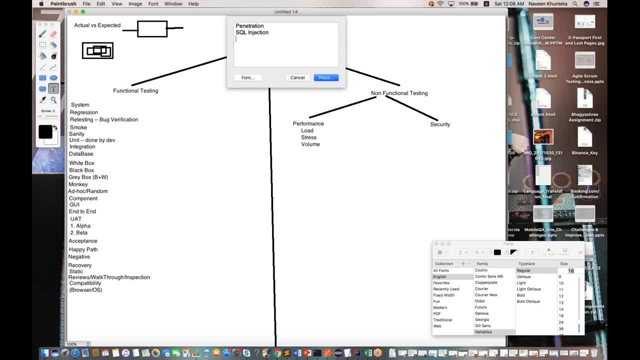 make sure that your security testing is okay, happening properly, all the one vulnerability testing. you will check, okay, that hacking and all those stuff at the network layer, at the client layer, at the database layer, at the server layer. you are checking that. okay, that your data should not be accessible. 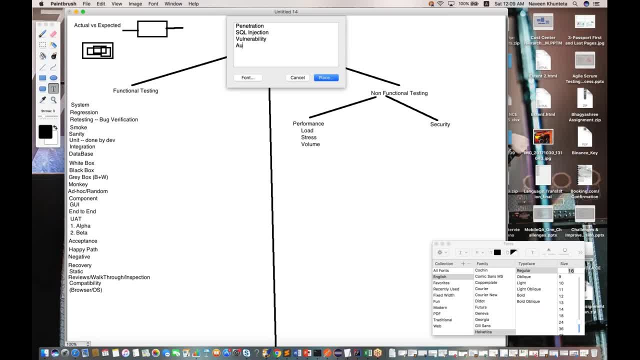 authentication authorization: okay, authentication, username, password, password should be in a strict form, masking form, okay. so such kind of things you will be checking. with respect to security testing guys, okay, so that's why, like these are different, uh, you know, types of testing: functional testing and non-functional testing. 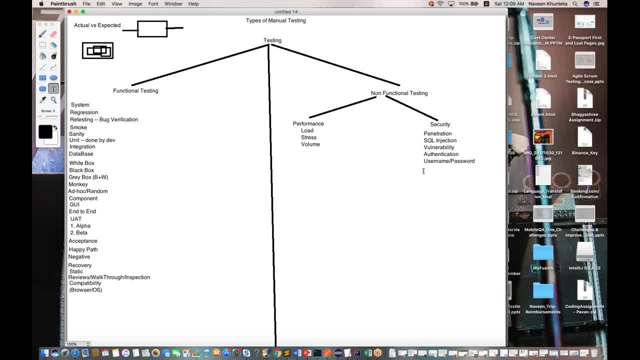 so, if you compare, like, what do you mean by manual testing? so, as i told you, manual means actual versus expected, but all the things you are testing manually, you have to write the test cases for that. so the first thing is that you have to write the test cases. okay. 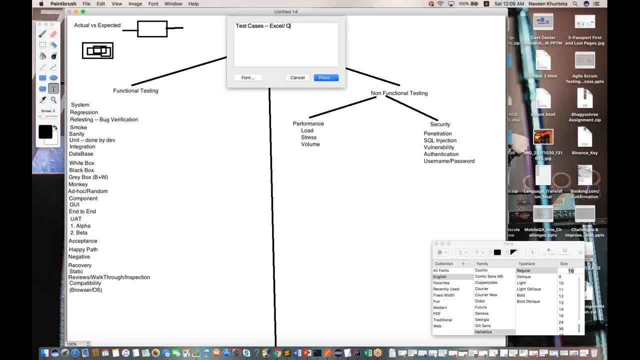 maybe in excel file or maybe some quality center tool, some tool you have to use, or maybe different tools are available. test rail is there? the different test cases you are writing, but all the test cases you will be writing manually. okay, manually. there are no automation. you are writing for that, so manually you are writing your test cases. some myth about? okay. 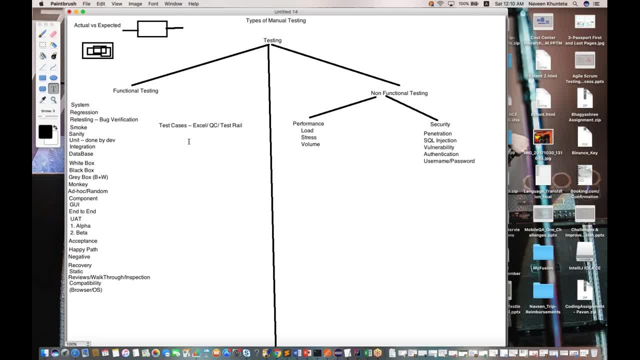 there are some myth about manual testing. okay, i would like to highlight those. first thing is that anyone cannot do manual testing. it's not like that. okay, any guy can do manual testing. you need some extra skills, okay. so okay, you need to know how to design your test cases. what are the positive- negative scenarios? you have to write different type of. 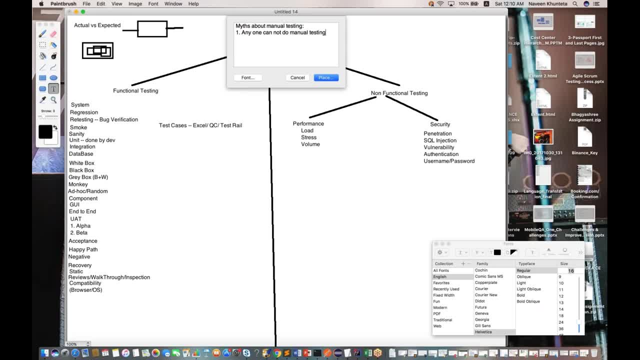 like boundary value, and this is different type of techniques you must know. okay, to become a manual tester, okay. second thing is that you should have constructive mind, guys. constructive mind with destructive approach. that's very important, that your mind is very constructive. with destructive approach, you want to break the system. 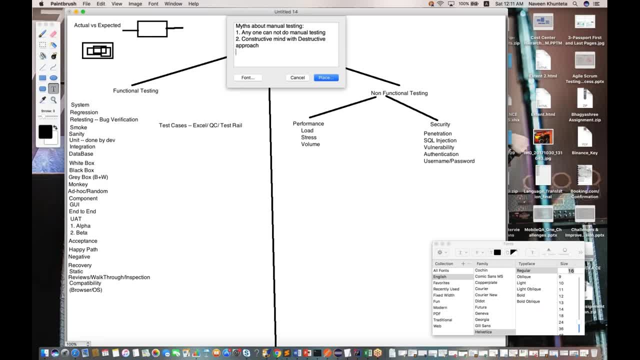 okay, you are. okay, you want to break the system. you are checking the application end to end, with all the positive and negative scenarios. okay, that, with the proper destructive approach. you want to break it, but with the proper constructive, systematic approach. third thing is that if you don't have such kind of skills, you cannot do that. okay, anyone can do that. no one, it's not like that. 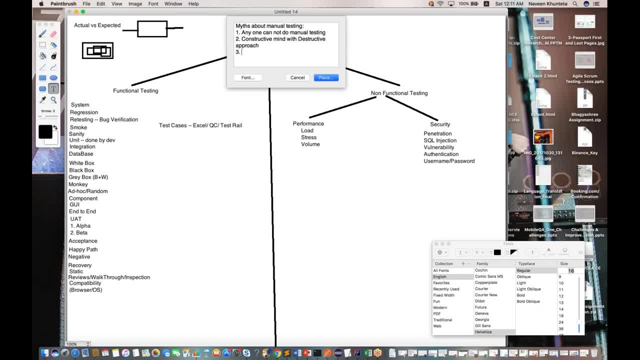 okay, any guy can do manual testing. third myth is that if you don't have domain knowledge, okay, if you don't have no domain knowledge, or maybe without domain knowledge, you can do testing. no, without domain knowledge you cannot do that. you must know what kind of application it is okay, what kind of product features are available. then only. 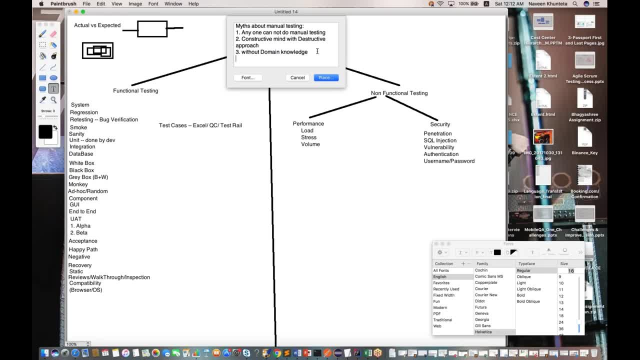 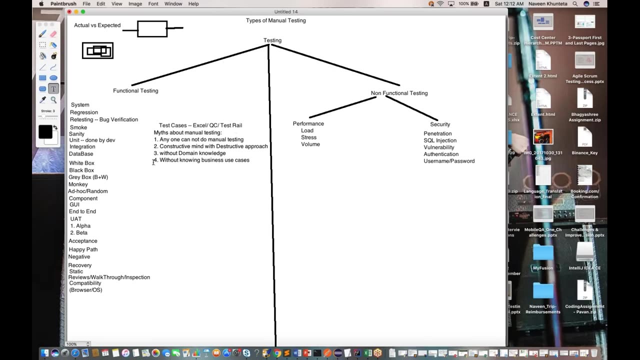 you can do that. so without domain knowledge you cannot do that. you must know that. okay, what are the different? without knowing business use cases? so without knowing business use cases you cannot do such kind of manual testing. okay, and some myths are available, that okay, one more myth is there that is: uh, okay, that is called. 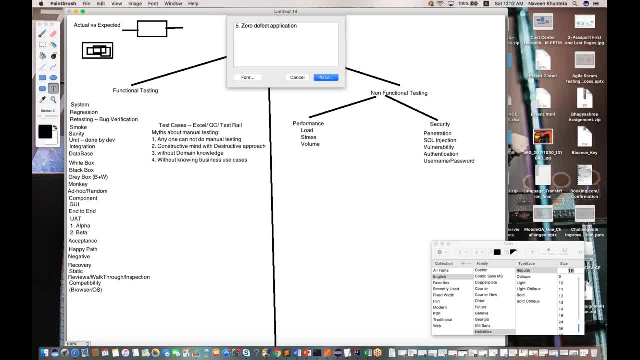 zero defect app application. so you guys, it's not possible that only you can find each and every defect in that particular application. it is not, no one can find it. any application cannot be 100 percent bug free application. zero percent defects are there? zero defect application is not possible. you are checking. 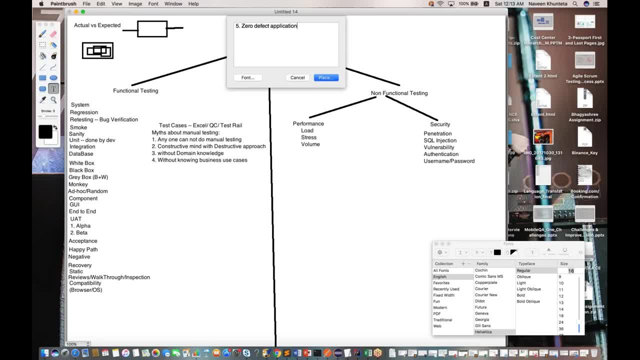 that particular application from last five years. tomorrow, if i'm checking, i can fight ten different issues in that particular application. that is true. okay, just accept it. zero defect application is not possible. okay, there are some issues. there will be issues always. some use cases, some special use. 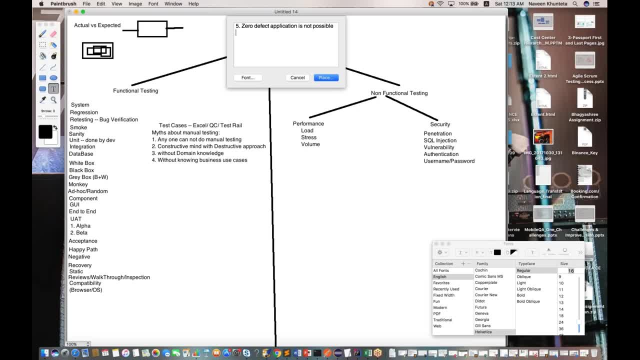 cases or corner cases. you have missed, you haven't thought about it. okay, you will be realizing once the use cases are done by the, okay, by the customer, the actual customer production issues are there, then you will realize, okay, okay, this is what it is happening, but we always try our best to cover. 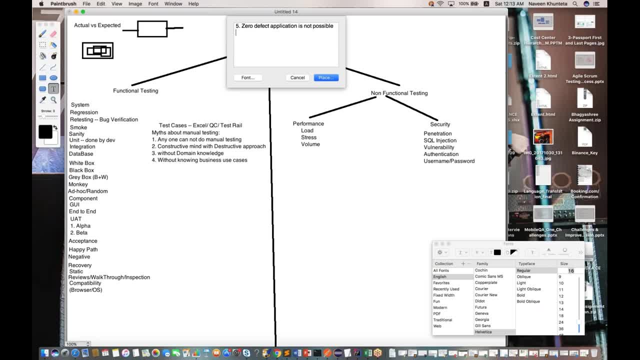 as much as possible. okay, so this is the thing that. okay, zero defect application is not possible. some myth about testing is that again, okay, so this is one of the myth. okay, so now, if you compare manual versus automation, so manual versus automation, it's very simple that. 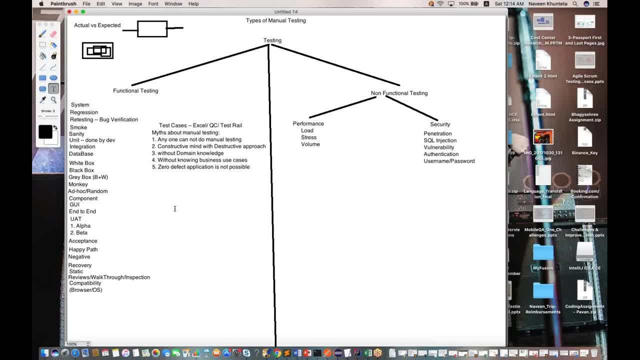 okay, in manual testing we write everything in the form of test cases manually. we have to write without automation code. but in automation we have to use some tool, like we have selenium quality, qtp we have. we have a lot of other tools. we have to use some tool, like we have selenium quality. 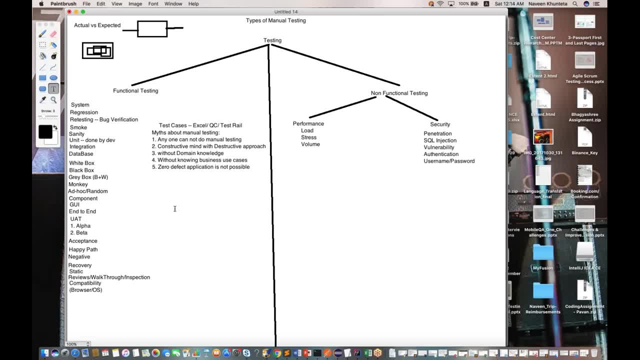 we have a test complete performance testing point of view. we have load generator diameter swap, uie for back-end testing srtp client. so we have to rest assured such kind of things we have to use for different types of okay testing. either it is function testing or non-function testing. but 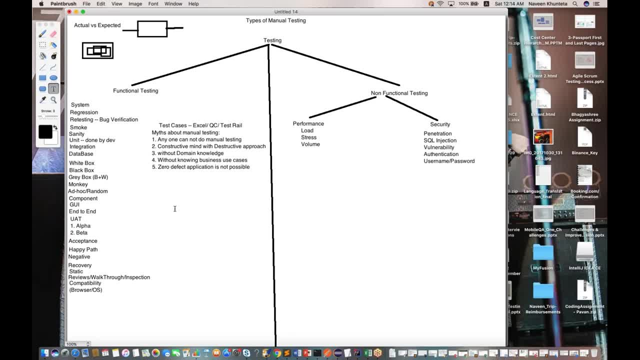 we are using some tools and we are writing some code, okay, so that we can save a lot of time. so manual testing obviously it's a time taking process and sometimes it's boring. it's a similar kind of job you have to perform again and again, so that's the biggest challenge, okay.